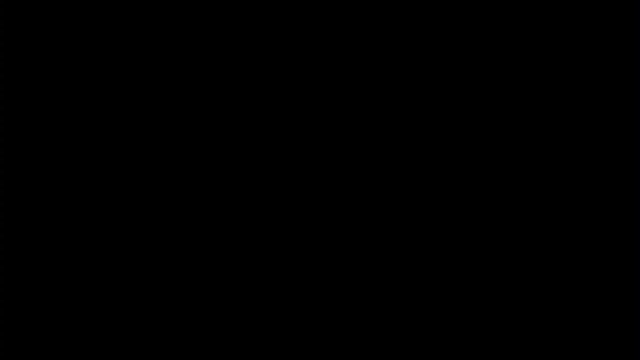 probabilities and it's all about what the probabilities are of certain particles. so let's say we have some particles here, um, just sort of whizzing about- doesn't necessarily have to be a you know, they're just sort of whizzing about, um, they might have this amount of energy or they. 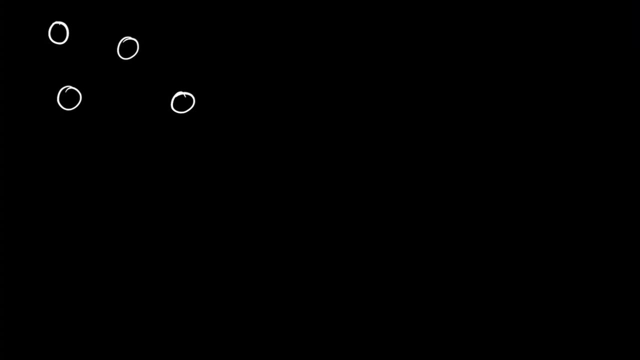 might have this amount of energy, or they might have this amount of energy. we really don't know. but what you can do is apply, probably, a probabilistic approach, so like be able to tell what the probability is of a particle having a certain amount of energy and we call a certain 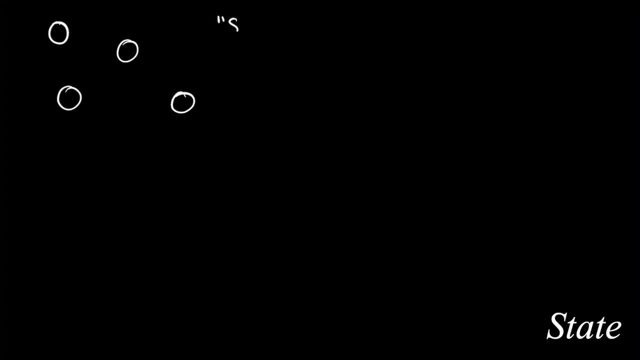 energy level. we call it a state, and a state is a pretty important word when it comes to statistical mechanics. you need to know what a state is. it's basically a energy level. so, for an example, say you have an atom with his own nucleus and you have electrons whizzing around the atom. the electrons can occupy certain states. 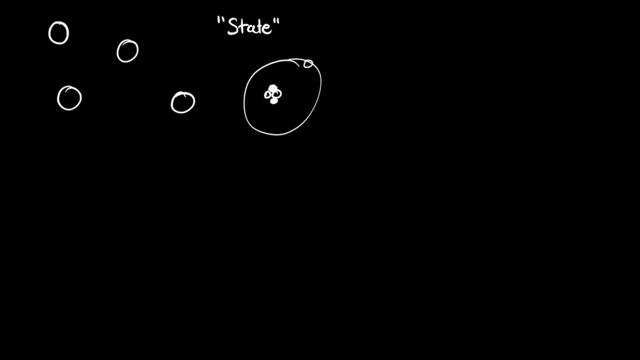 and so if it's, you know, in the shell that's closest to the nucleus, then it has this energy state. if it jumps up one, it has the next level up energy state. of course, quantum mechanics tells you that these states are quantized, and this is what basically a state is: it's an energy level. 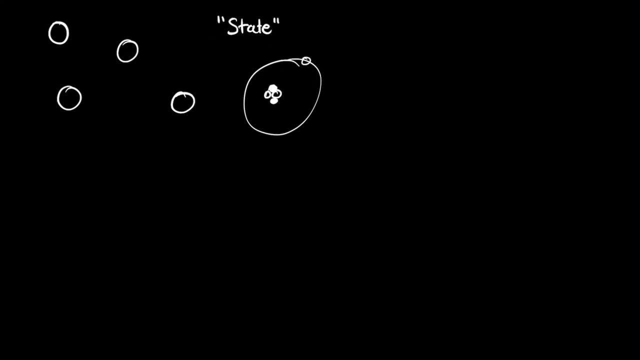 and the way we like to kind of represent these states a lot in physics is you have, uh, sort of like a ladder, almost, so you've got to kind of imagine a, a completely artificial ladder, and the rung of the ladder represents a certain energy, um so let's just call this rung, let's call this the. 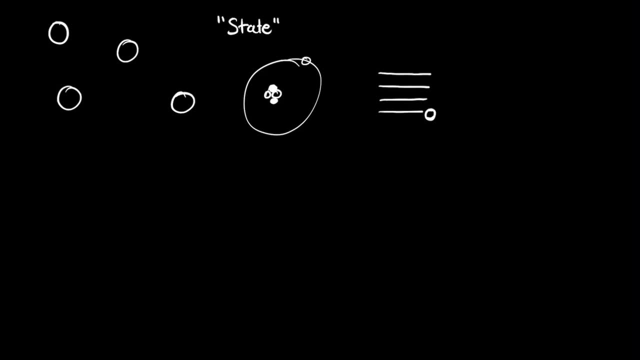 zero energy state. so what I mean by the zero energy state is if a particle has absolutely no energy at all, then that's the zero energy state. um so, but what about this one right here? well, let's call it a name. we could call it anything. let's call it Epsilon. um, Epsilon is a certain amount of. 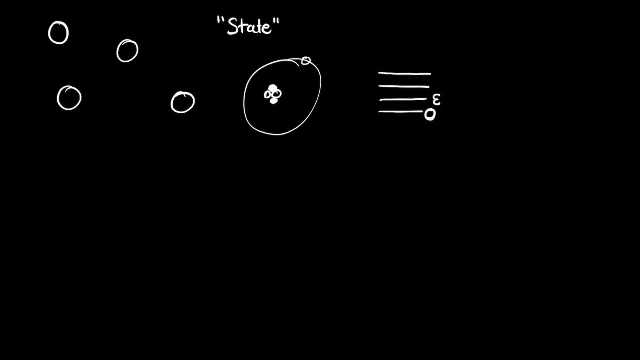 energy, uh, that that a particle might have. um, so, moving up, you can have two Epsilon, three Epsilon, Etc, Etc, and you could go on potentially forever. um, in classical mechanics, there's no restriction on how many energy states you can have. uh, for a certain, for a certain system. 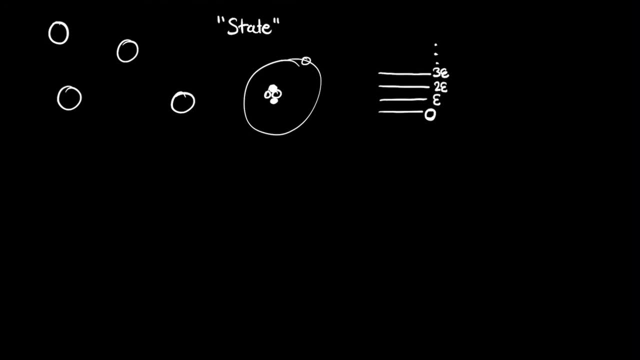 um, normally the higher energy states are much like less likely to be occupied, and that's one of the things that statistical mechanics actually predicts quite beautifully is that high energy states are less likely to be- uh, to be occupied, which is probably a good thing. considering like high energy states, you know, if things, if particles, have a lot of energy, then you know, we're kind of a. 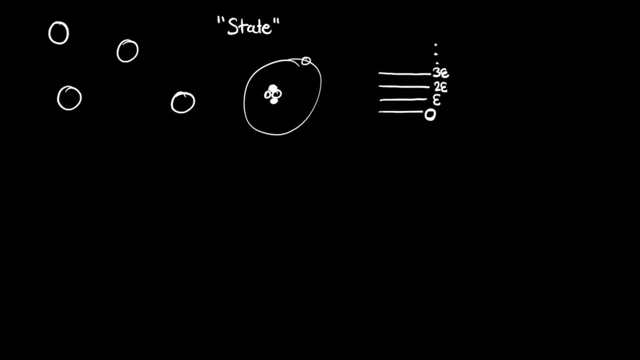 bit really, because then you know, we'd kind of have, you know, x-rays coming down from the sun, and statistical mechanics does predict that these high energy states are less likely to be occupied. so here we go. this is going to be our basic model, for this video is our kind of set of, our set of. 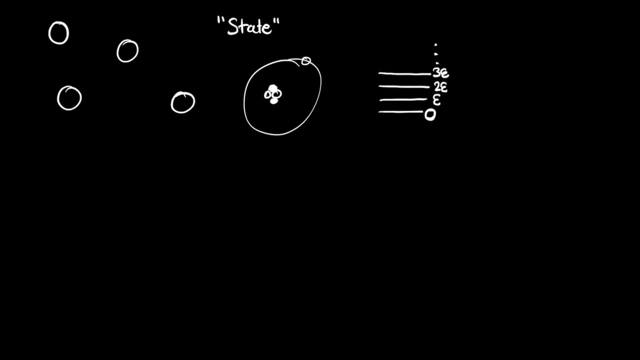 energy states. so let's do a simple example. um, let's take the simplest possible uh example. that's very easy to explain. um, now we're going to have three different systems. I'll draw them in different colors so you can see, uh, which ones they are. so let's have system a right here. 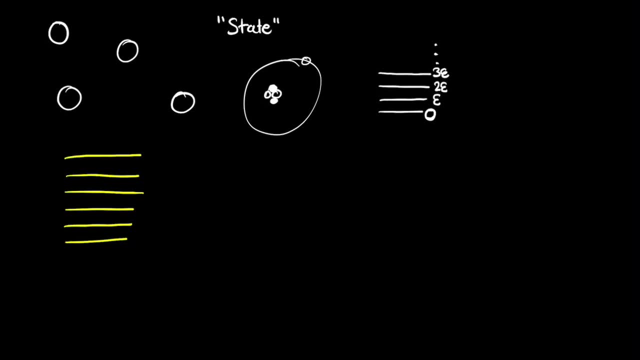 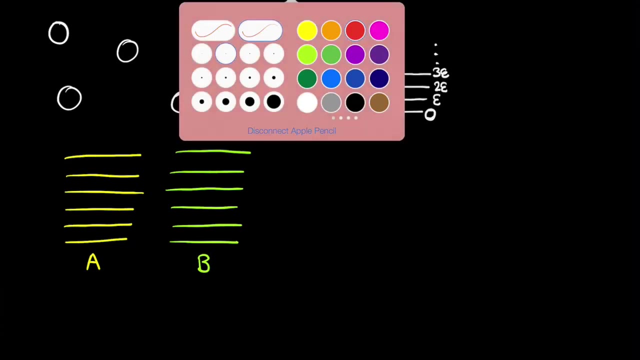 and these systems are absolutely identical. there's no difference between them. so let's just call this system a. we're also going to have an identical system. I'm gonna have system B, and what I'm drawing here is I'm essentially drawing the energy levels of each system, so 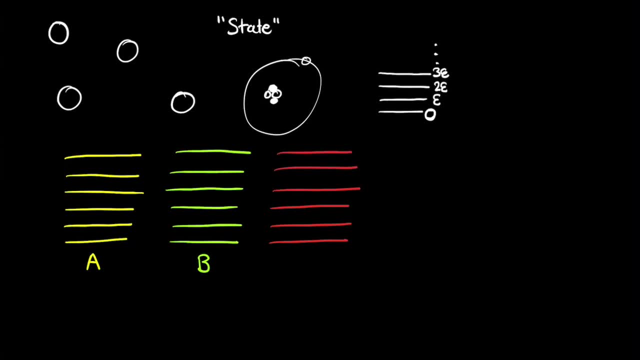 it could be, say, three pendulums or three boxes of gases, but the point is that each of them has a certain set of energy levels which they could occupy, and this is system C right here. so let's say each system has one particle in it and this particle, it could be anything, could be a proton. 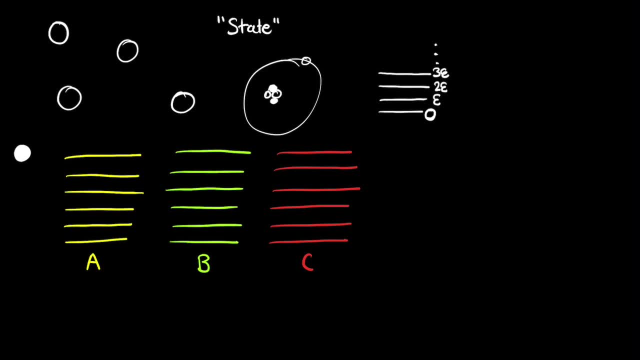 it could be an electron, it could be a neutron, it could be an anti-quark plasma glue or neutrino or whatever the crap it that is. I think I just made that up, not gonna lie. and this particle? the point is is that it can only have. 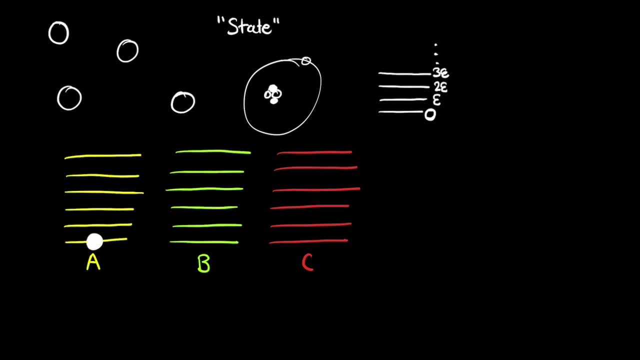 these energy levels. it can't exist in between. it can only take a certain energy level. um, and we're going to ask: what is the probability of a particle being in a certain energy level? now, uh, we're going to firstly say that let's just let these energy levels go on forever. um, you know, in all three of 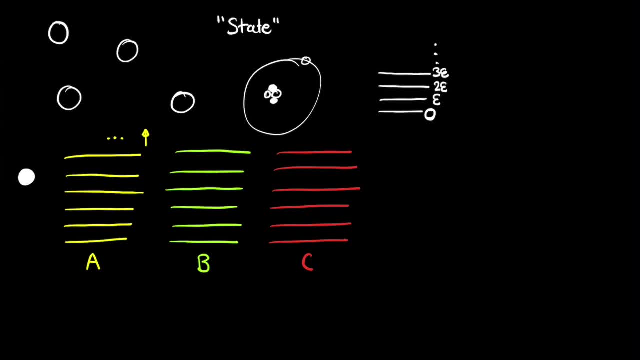 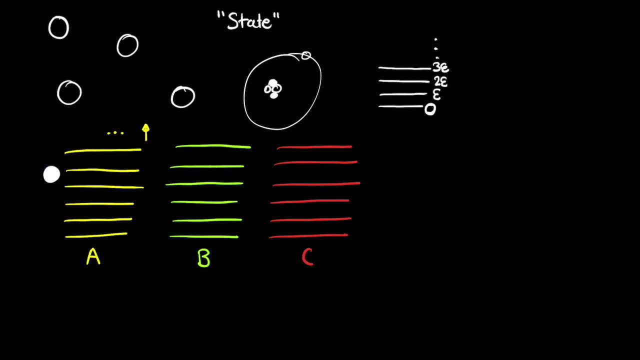 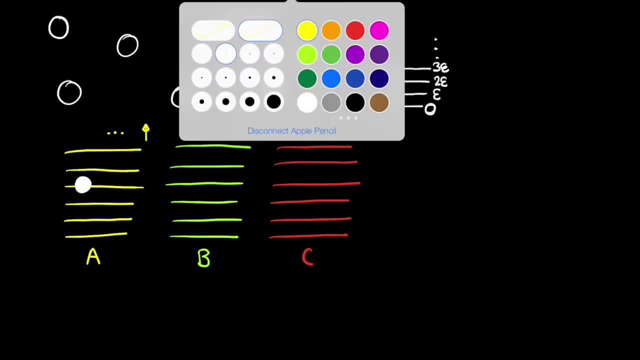 these: uh, in all three of these systems the energy level just goes up and up and up forever. um, but it doesn't really matter. but let's say, for example, system a has this particle up up here, up on this energy level, right here, in fact. let's just make this easier and give these, um, give these little. 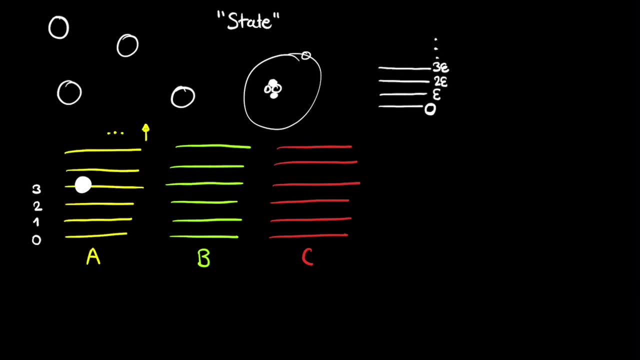 numbers right here, so naught one, two, three there. we're not going to bother with units, but if you want, you could attach some units if you wanted to. uh, but this just shows the. you know quantization right here. um, so system a has this particle up on level three. uh, what about system b? well, let's say, 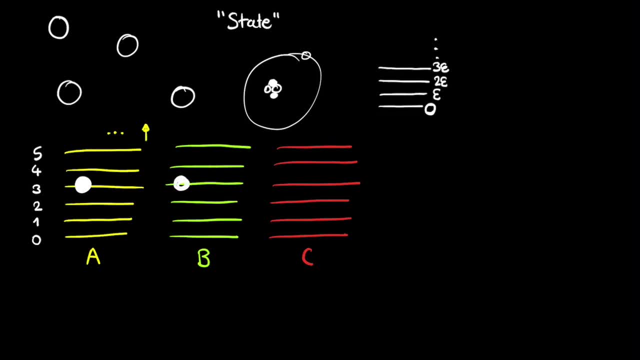 that system b also has it on level three and system c has particle on level zero. and so we're going to ask ourselves the question: how many possible ways of distributing a certain amount of energy? so let's say we have a certain amount of energy, um, let's call it six. uh, so say we have six units of energy, how can we distribute these six units? 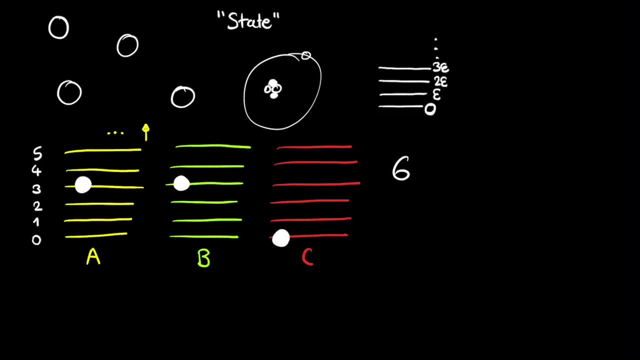 of energy throughout these three systems. um, I'm going to assume that these two systems are what's called distinguishable, and we'll come on to what that means. um a little bit later on, because this concept actually becomes very important. um, when it comes to quantum mechanics, because quantum 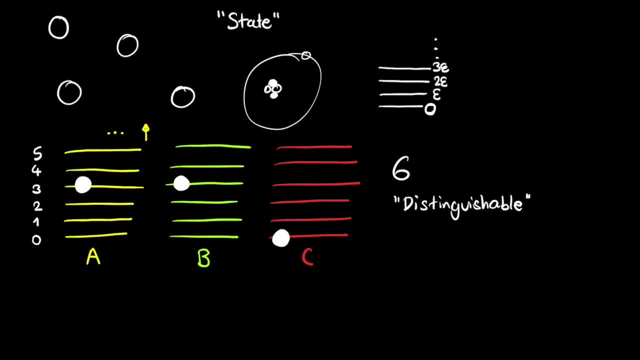 mechanics of uh. you know quantum mechanics of uh, you know quantum mechanics of uh, of energy says that particles are fundamentally indistinguishable. but for now we're we're still in the classical realm. we're going to assume these particles are distinguishable. so yeah, how many ways are there of distributing six units of energy amongst three systems? well, 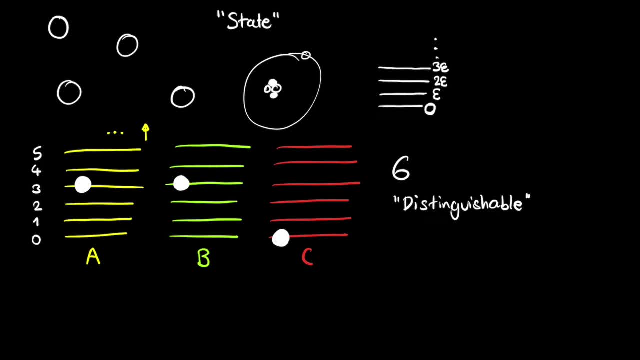 that you could count them all out if you really really wanted to. but, uh, we kind of want it to do a a little smarter way, to be fair. but before we work that out, we're just going to introduce a term, um, and we're going to introduce a term called micro State. this is quite an important term. 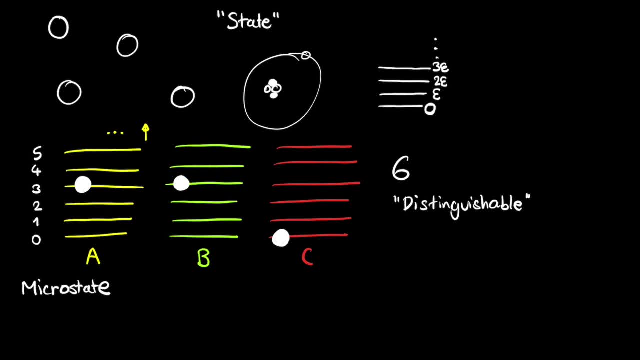 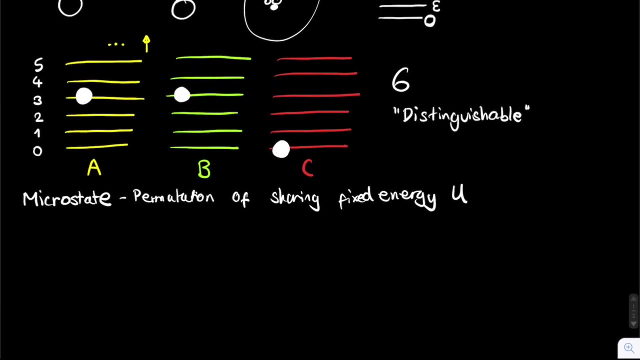 um, when we're when we're, when we're talking about thermodynamics, and what a micro State is, is a permutation of sharing a fixed amount of energy. let's just call it you for now, and so this is what a micro State is, and I've actually just drawn a micro State right here. um, you know, one micro State. 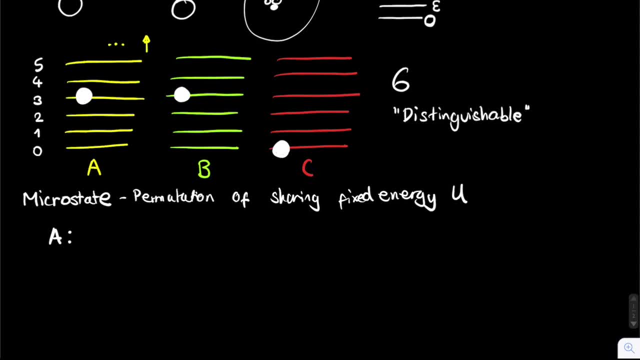 has this state that i've drawn has system a with three units of energy, system b, also with three units of energy and system c with zero units of energy. now, the key word here is permutation. i've not written combination and there's, and you need to understand the difference between permutations. 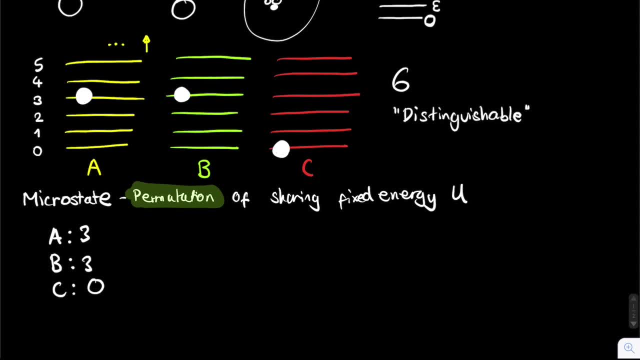 and combinations and, if i'm honest, i actually thought that they were exactly the same word for quite a long time, which was not a great thing, because when it came to statistical mechanics, i got very confused. so before i go any further, i'm going to tell you what the difference is between. 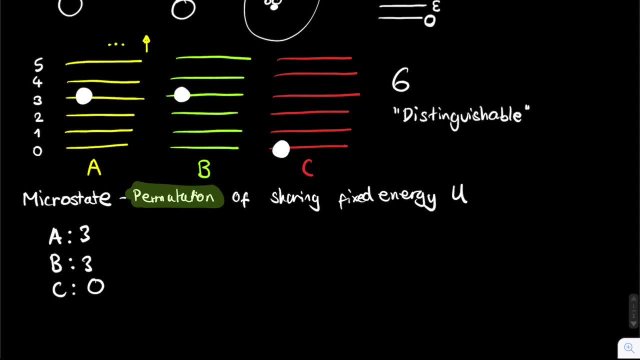 a permutation and a combination is. so let's say, let's take a really really, really simple example. so let's say, you've got the numbers one, two, three, a, a permutation in a permutation. the order matters. so: one, two, three, how many different permutations, permutations are there, how many different ways are there of ordering these three numbers? well, 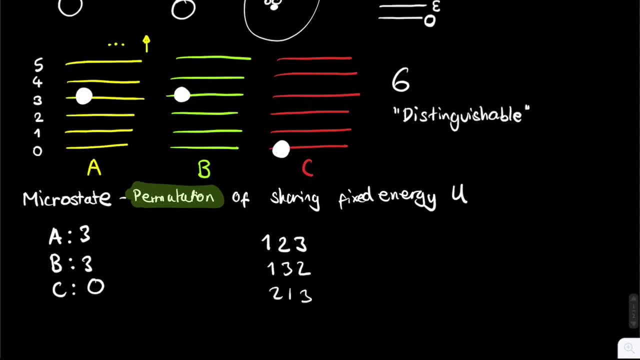 you're gonna have one, three, two, two, one, three, two, three, one, three, one, two and three, two, one. so there's six permutations, aren't there? uh, six different ways of ordering, uh, the numbers one, two and three, and what is a combination? uh, well, the combination is still the same. uh, you've got. 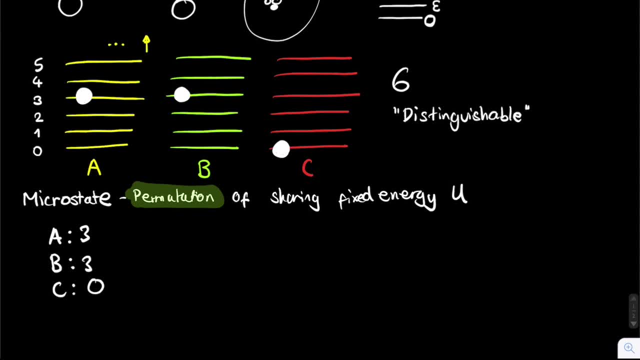 exactly the same uh numbers, you know: one, two, three, so that just counts as one combination, uh, and so you can say that there's six permutations for this particular combination. a different combination would be one, two, four, uh, and again you'd have six different ways. um, take a, maybe a four digit number, you know. 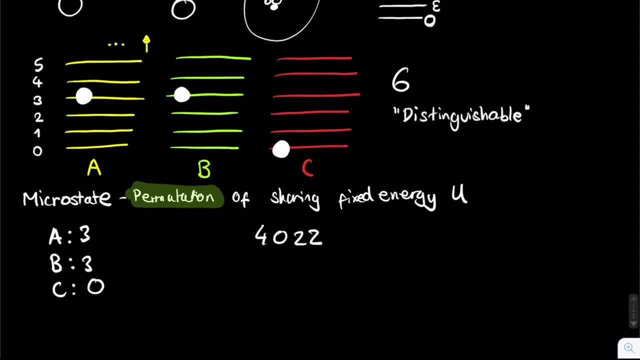 four zero, two, two. what have you got? you've got two twos, a zero and a four. um, to be honest, i can't be bothered to work out how many different permutations are there for this particular combination. you know, basically one combination for every number, so you have to apply a combination in order to actually 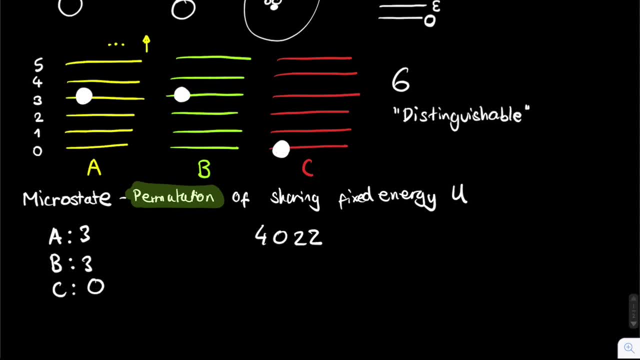 you know, to 20 or 20 words and you see that comes out in there. so that is basically what the difference between a permutation and the combination is. think about it. you know, maybe if you're playing a game of cards, each poker hand is essentially a combination. 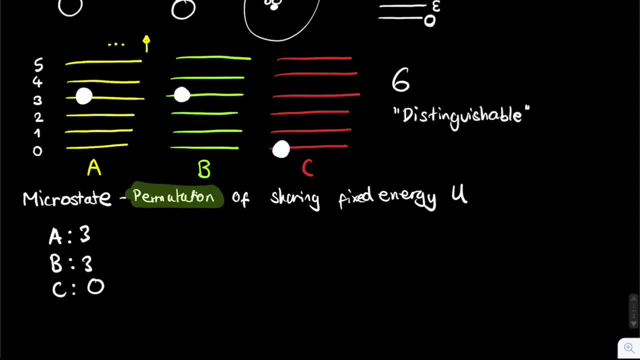 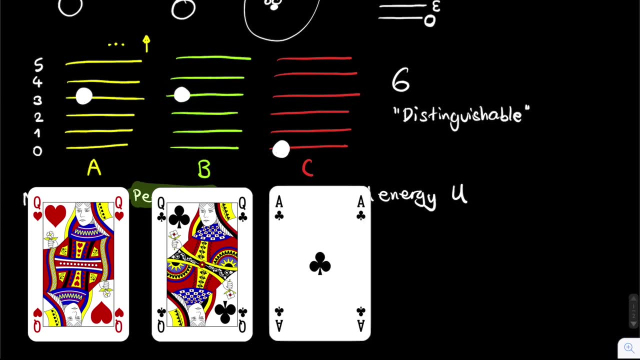 because it doesn't really matter what, what with order you have your cards in, does it? you know? it doesn't matter if you have king queen jack, queen ace, you know, or queen queen ace jack king, yeah, it doesn't really matter. that's the combination, but if it's, if you're talking about, 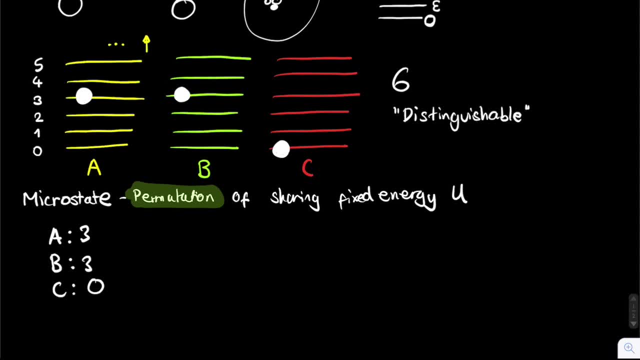 permutations, then you obviously have, you're going to have many more permutations than combinations. so always remember, permutation is the bigger number than combinations. so that is what a difference between a permutation and a combination. and a microstate is a permutation of sharing a fixed amount of energy. you, so i've drawn out one microstate, this 330 microstate we can just give it. 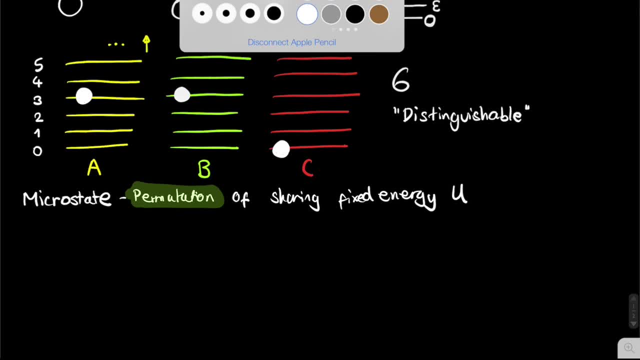 a temporary label. we can just call it um. you know 330 right here and you can probably go through and work out all the different microstates of sharing this amount of energy. and if you do that, in this case you've got three systems and you're distributing six units of energy. then you'll 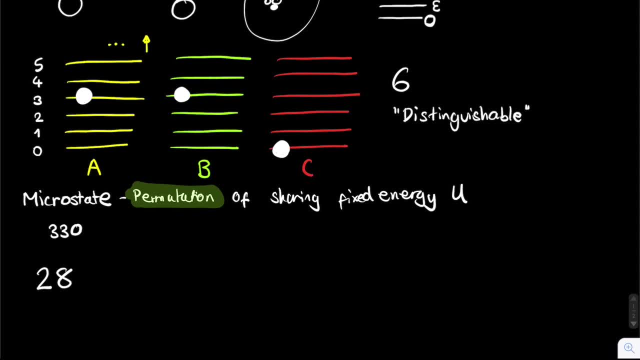 actually find that there are 28 different microstates and we call the number of microstates, we give it the symbol omega and we just simply put a little subscript, n? u, right there. n is the number of systems, or the number of particles, if you want, and will become the number of particles when we apply this. 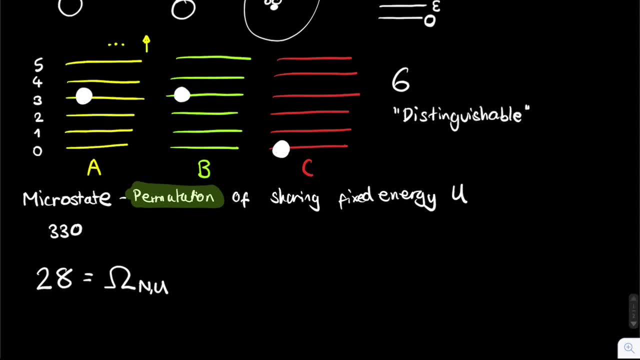 to thermodynamics and u is the amount of energy. so in this case n equals three, u equals six. so that's the number of microstates. we give it the symbol omega and we just simply put a little. so you guys are probably wondering: how do you get 28 out of three and six? you know how on earth did. 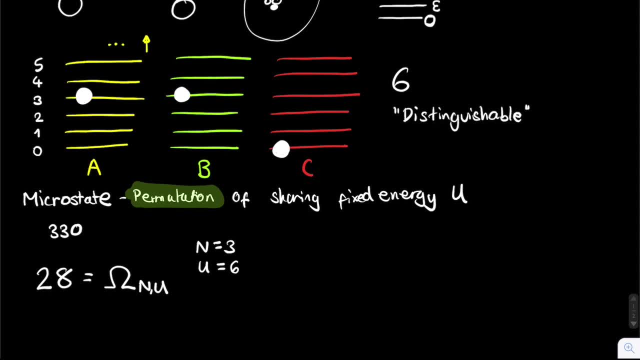 you know that it was 28. well, there is actually a formula which, again, i'm not going to derive um, but it's a pretty useful formula, and it is given as the number of microstates, omega and u is given by n plus u, minus one choose u. so this is a bit of statistical notation. uh, you guys probably are familiar. 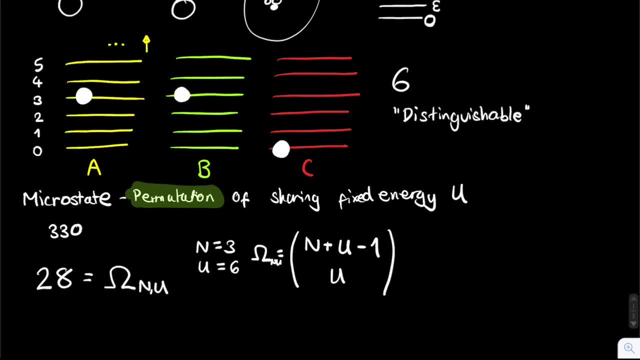 with what this brackets is. it's basically the binomial coefficient. it basically means n plus u minus one, all factorial over u factorial multiplied by n plus u minus one minus u factorial. so remember, six choose two is equal to six factorial over two factorial times six minus two, which is just four factorial, and that's the binomial coefficient. it's. 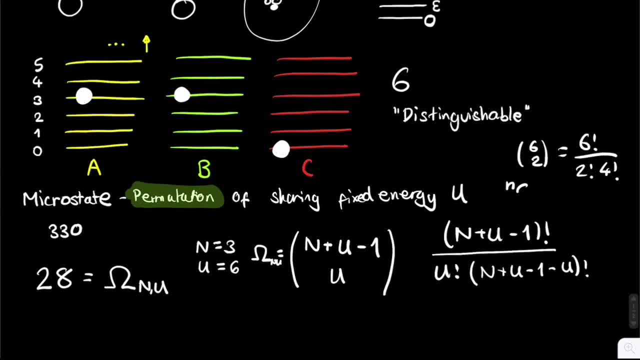 the um, n. it's often called n, c, r, right there, that's what it is in maths, but here in statistical physics, um. this is what the number of microstates is, um, and it's the. it's this formula right here, pretty handy formula. so actually, if you work this out, then in this case you, you're going to end up. 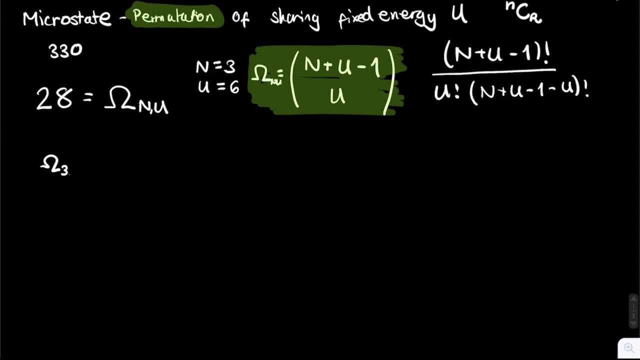 with omega 3, 6 is equal to well, 3 plus 6 minus 1. choose 6, which is equal to 8. choose 6, which is equal to 8 factorial over 6 factorial times 2 factorial, and you guys know what factorial. 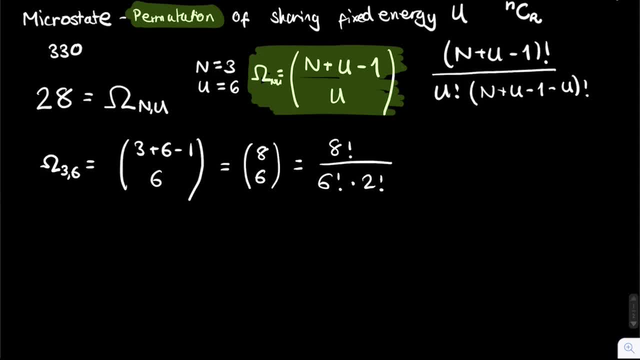 means right, it's 8 times, 7 times, 6 times, 5 times, 4 times, 3 times, 2 times 1, etc. etc. and if you do that, you end up with 28 being the number of microstates, and so that's quite a handy formula. 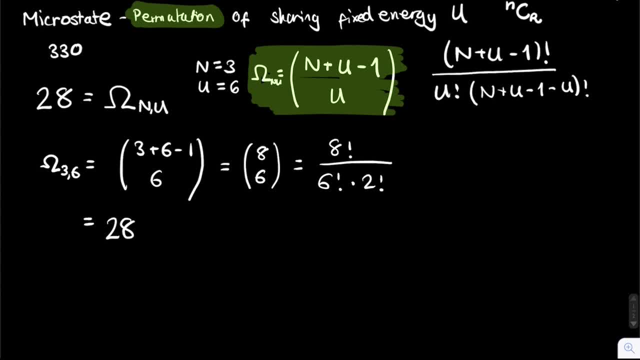 um, to work out the total number of microstates in uh at this system right here. so what's next? well, well, we're going to make a postulate right here- and we do this a lot in physics. we like to make our postulates- and we're going to say that all of these microstates, all of these 28. 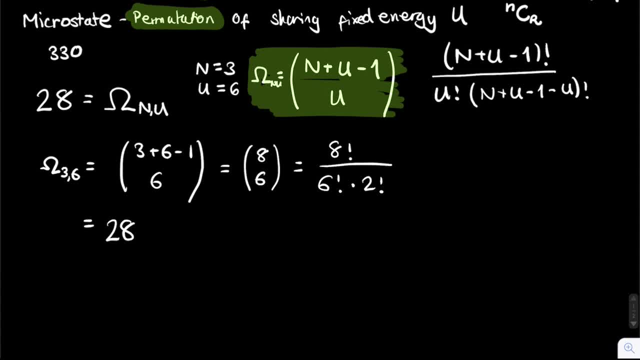 microstates, all of these 28 different ways of sharing this energy. u are equally likely. and so what? how are we going to write that? well, we're going to write that as p. where p is the of a system being in a particular microstate is equal to 1 over the number of microstates, 1 over 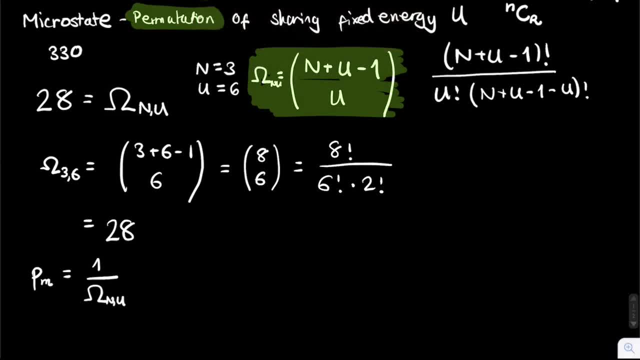 omega, which seems fairly obvious. you know, there's no, no bias. so we can assume, for the moment at least, that the probability of the system being in a certain microstate is exactly the same for every different microstate. so that's what we're going to write. that's what we're going to write. that's. 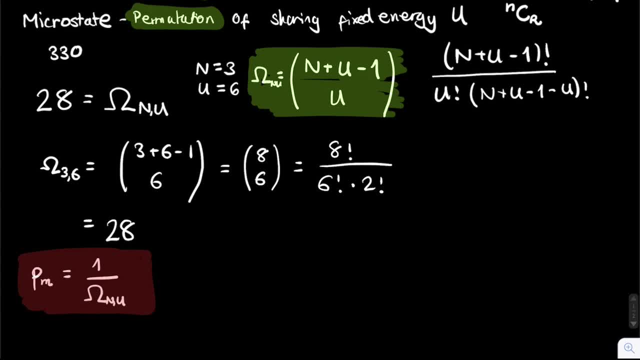 what we're going to write. so you know, 3 3 0 has exactly the same amount of probability as the- i don't know- 4 1, 1 microstate, or the 5 0, 1 microstate, or the 3 2, 1 microstate, you know. 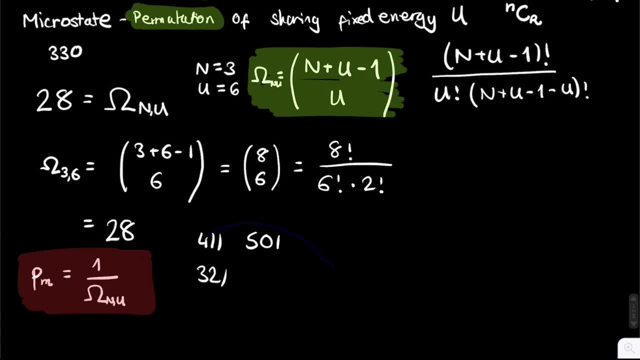 they're all equally probable. all the 28 different microstates are equally probable. now, as is the case with a statistical- uh, a statistical- approach, there is one thing that comes up a hell of a lot you need to know, and that's pretty important, and that is that every single possibility, the 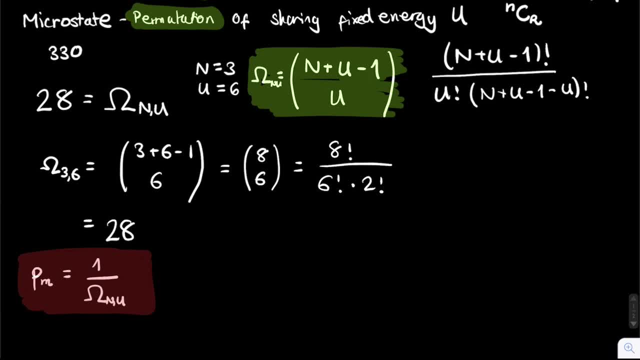 probability of every single state must always add to 1.. so that must mean that the probability of every different microstate must always add to 1.. so in this case, we've got 1 over 28 plus 1 over 28, plus 1 over 28. how many 1 over 28s are they going to be? well, there's going to be 28, obviously. so if 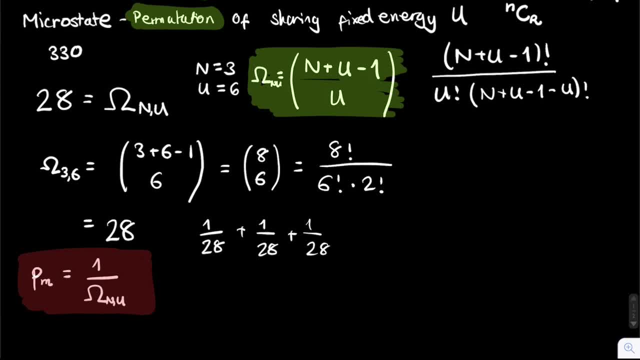 you add 1 of 28, 28 times, you're going to get 1, so all is well. but that's a pretty important thing and it's called normalization and that is the condition for any sort of probability. any time you talk about probability, you must know that the sum of all probabilities, the sum of all probabilities, 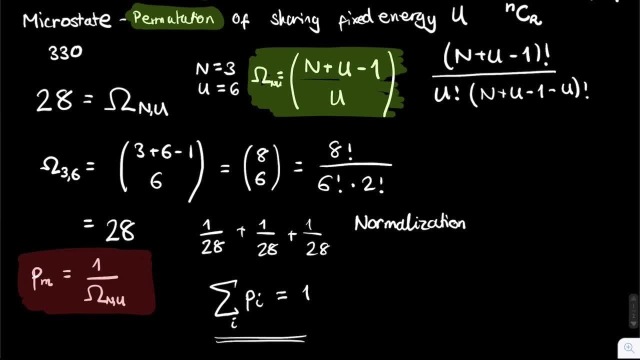 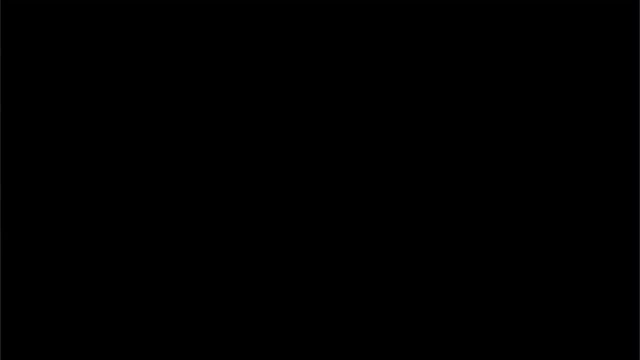 must equal 1.. that's very, very important and we'll be using that condition a lot to derive lots of useful cool stuff. so that's a little introduction to statistical physics. but i'm actually going to go back to entropy and i'm sort of going to parachute in an equation that might look a little. 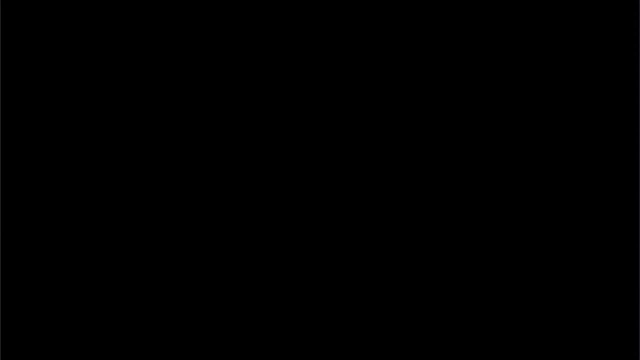 bit weird for the moment. i might be a bit weird to introduce this now, but it will become very clear how, um, how, this definition, that this starting definition, ties in quite beautifully with thermodynamics and it. you guessed it. it's all about entropy. we are going to define a statistical definition for entropy. now you remember what i? 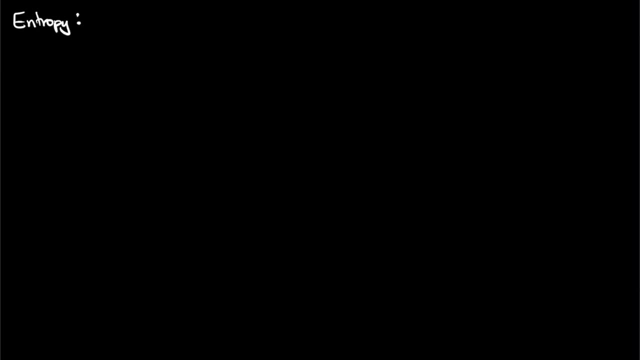 said about entropy. in one of my thermodynamics videos, i said that it's actually a measure of disorder. it's actually a measure of the amount of disorder, and so what can we call, uh, disorder? well, there's a number of different states. there are that you have of a certain system, the more different. 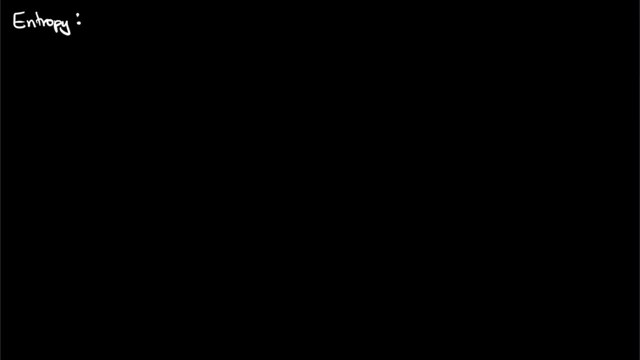 microstates the more disordered. and so what boltzmann did? our old friend boltzmann, who we're going to be talking about a lot? he defined entropy to be the boltzmann constant multiplied by the natural logarithm of the number of microstates. so you're probably thinking: what the hell? why have you? 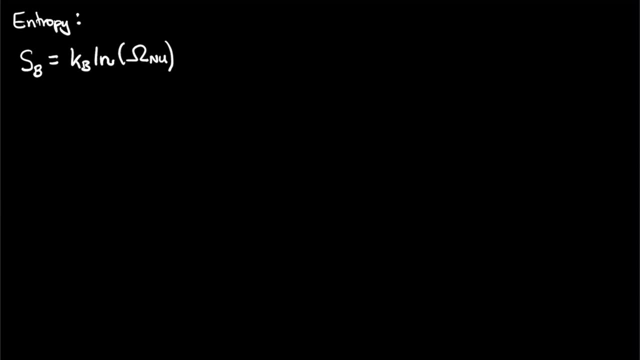 just written this. well, boltzmann did derive it. but we're actually going to start with this uh definition of entropy and we're going to sort of work our way back to thermodynamics, if you like, and we're going to work out how we can get from. 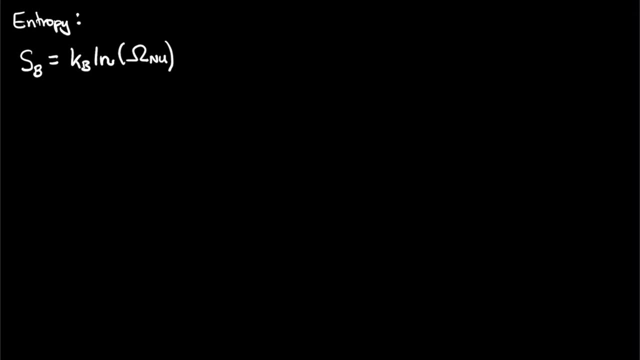 the entropy, uh back to what the we thought the entropy was, back in thermodynamics, which is, of course, uh, changing heat divided by temperature. so this is just a definition for now, and so basically the important thing is that this is just a constant right here, um kb, which is of course 1.3. 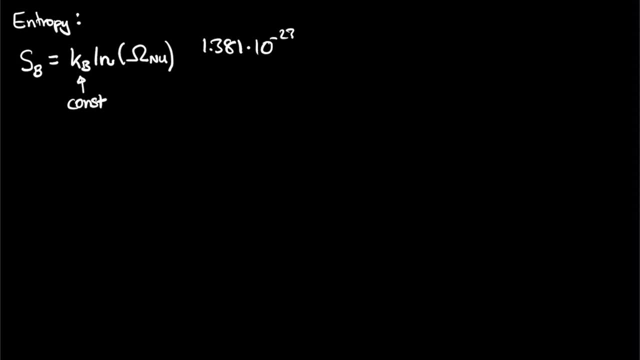 8, 1 times 10 to the minus 23. it's also there just to keep the units all good, and so it's the. the entropy is the, basically the number of different microstates of a system. so this is just a definition, and we this is actually what's called statistical entropy, um, and we're going to actually 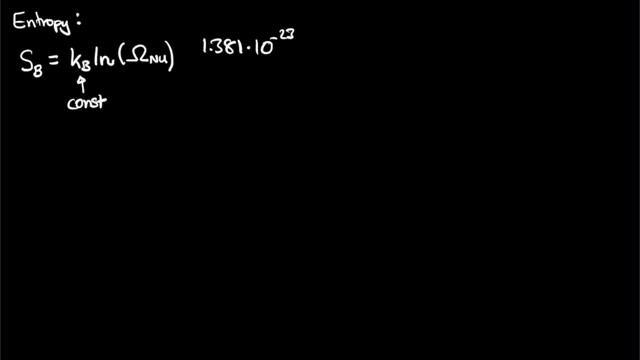 show a bit later on that it's exactly the same as thermodynamic entropy. uh, it's just two different ways of representing essentially the same thing, uh. but yeah, this is just a definition we'll work with for now. so we have a few problems right here. it's actually very hard to calculate. 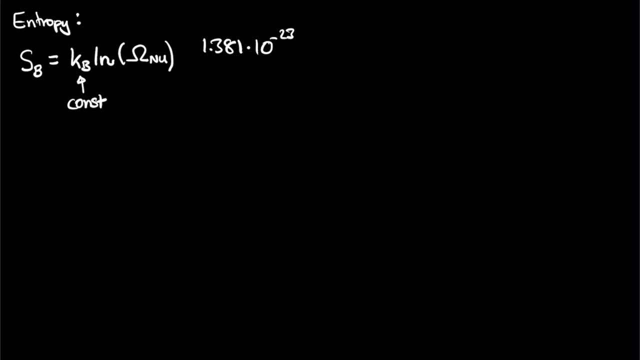 what omega is. i mean, i told you the formula before, but in a massive box of gas you can't possibly work it out all the time. it's very difficult to calculate. yeah, you just don't want to do it. basically, we're actually going to need to do some maths, uh, to get somewhere. a 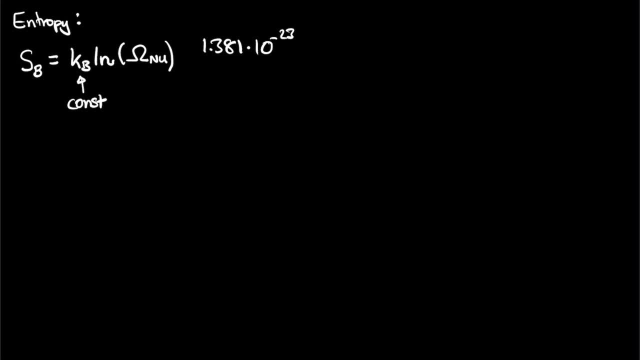 little bit better than this, uh, and secondly, it's also not reasonable to assume that the energy is fixed. um, you know, there are actually cert different types of what's called ensembles, and they're kind of a bit like what i was saying about, um, open systems and closed systems, uh, in. 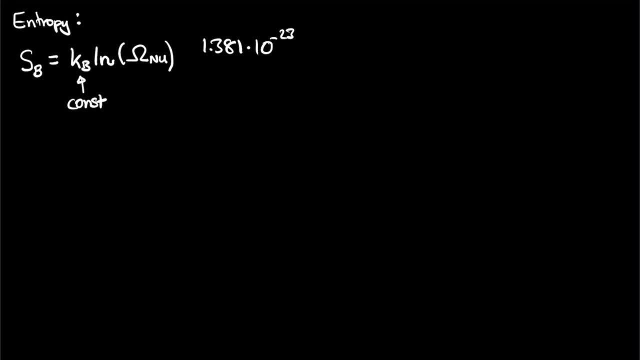 statistical, uh, mechanics. we call them ensembles. um, i actually i'll just talk you through the three types of ensembles. uh, that, uh, you'll need to look at in order to be able to calculate the energy that they are in. so far, are you have a set of energy levels, like? is that what you're looking at? 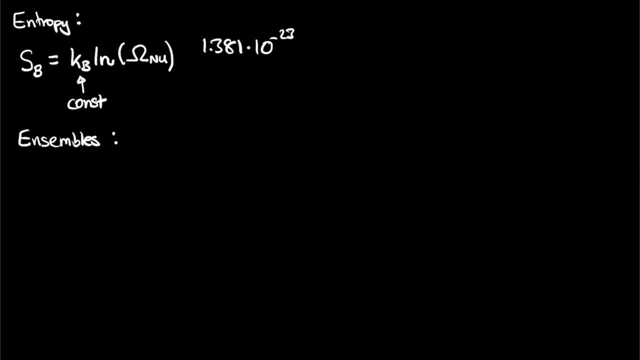 or are you using a system of state, like you're using a system of state that you'd probably need to know about. so, as i've just mentioned, essentially an ensemble is a system of state. basically, um, it's a set of energy levels, but instead of one, uh, you have several. so actually what i drew earlier. 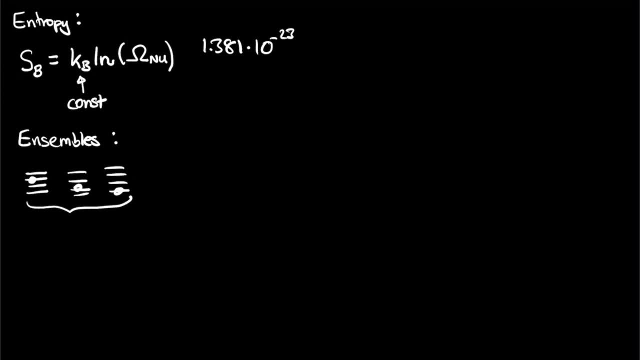 with these three different systems. this is actually what's called an ensemble. um, so it called an assembly as well. but yeah, basically it's a statistical way of defining what we defined before, basically a box of gas which can be either in contact with heat or particle bath or anything. 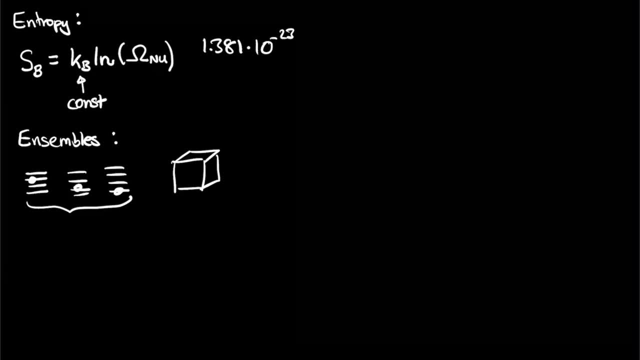 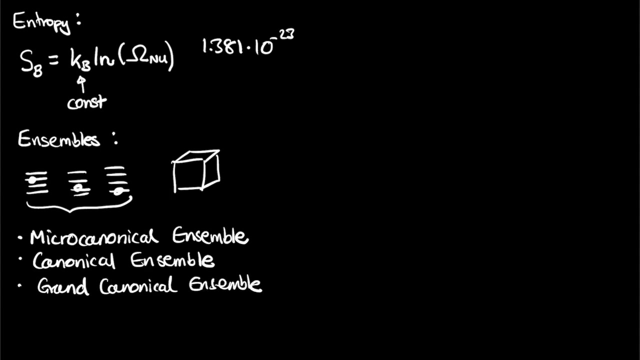 like that, but it's just. we call it something slightly different in statistical mechanics. and so what are the three different types of ensembles? well, there is the micro canonical ensemble, there is the canonical ensemble and finally the grand canonical ensemble. we're not going to come to the grand canonical ensemble for quite a while, but yeah, so these 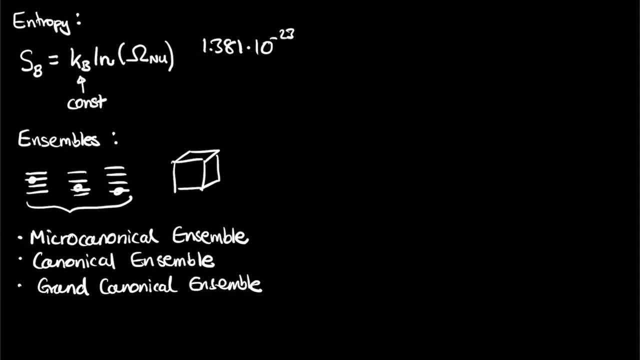 are three different types of ensemble and basically the micro canonical ensemble has a fixed amount of energy, the energy is fixed and it's basically analogous to a complete row ensemble, completely closed system in thermodynamics, which means that no temperature can get exchanged, no heat can get exchanged, you can't do anything. The system is completely closed. 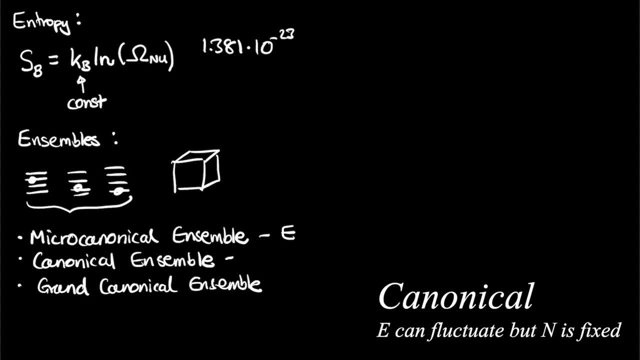 so nothing can get in or out. The canonical ensemble has a well-defined temperature at any point. It's similar to basically what we were talking about a lot of the time in thermodynamics before we allowed the particle number to change, And so basically, energy can flow in and out of the 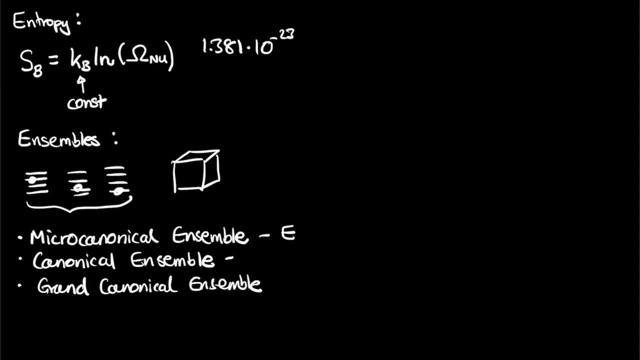 system, so the internal energy can change according to thermodynamics, However the particle number cannot change. That is the canonical ensemble And finally, the grand canonical ensemble. well, basically that is exactly the same as an open system and energy and matter can flow in. 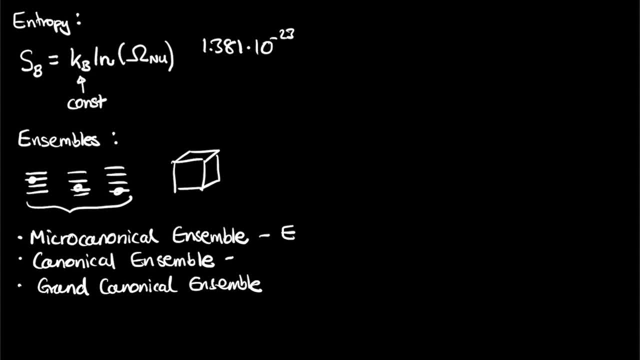 And the grand canonical ensemble is by far the hardest, and so therefore, we're going to come onto it last. But yeah, so that is basically the three different types of ensembles, and it's just a kind of fancy way of labeling the different types of system, basically. So what are we going to do with this Boltzmann? 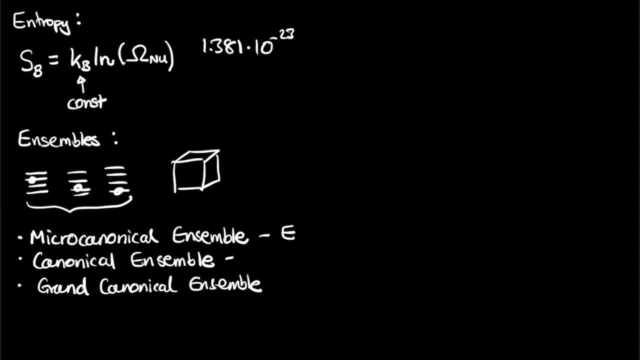 entropy that we've got right here. Well, we're actually going to make an approximation, And to do this approximation, we need to make another definition, And this definition is what's called a macrostate, And what a macrostate is. you might have noticed. 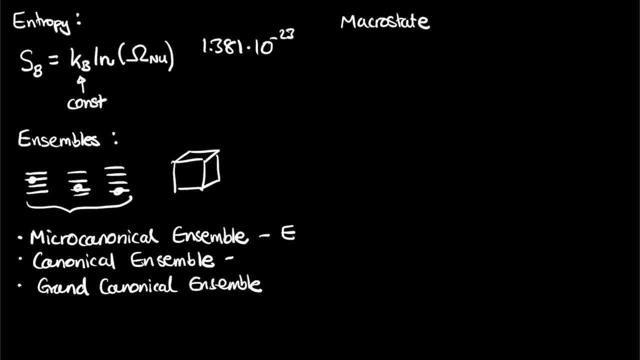 that a lot of these microstates that I was on about earlier so say, you have 033, you might notice that there are lots of different ways of ordering this set of numbers. So you could have 303, or you could also have 330.. Now 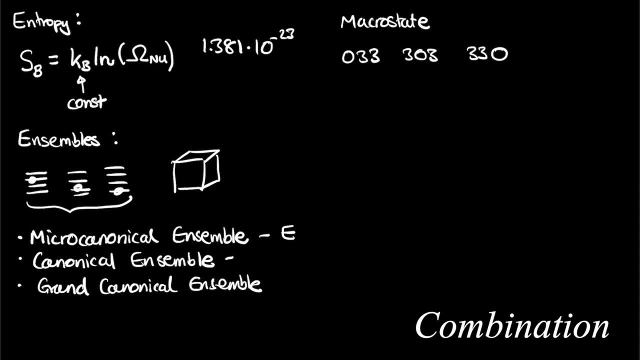 this is actually a combination. pretty much, The definition is very similar. A macrostate is just like a combination of numbers, whereas the microstate is, of course, a permutation, And so this right here is collectively one macrostate. It's the macrostate that has 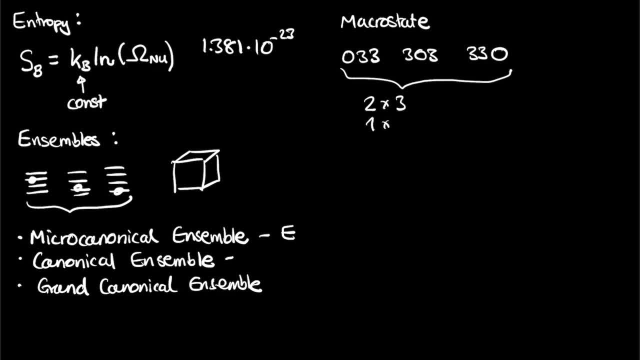 two lots of threes and one lot of zeros, And so that is how you kind of define a macrostate. It's a little bit harder to write than the microstate, But yeah, that is the macrostate, And we tend to give the macrostate multiplicity the symbol w, And so in this case w is simply equal to three. 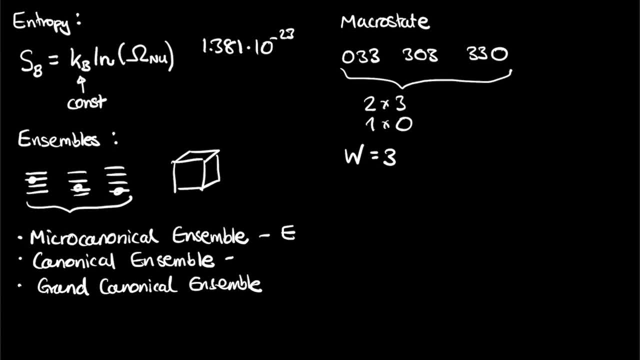 It's not the number of macrostates in total, It's the number of microstates per macrostate, if that makes sense. So in this case, right here, we have three different microstates, but we can see that they're all comprised of the same numbers, And so therefore, 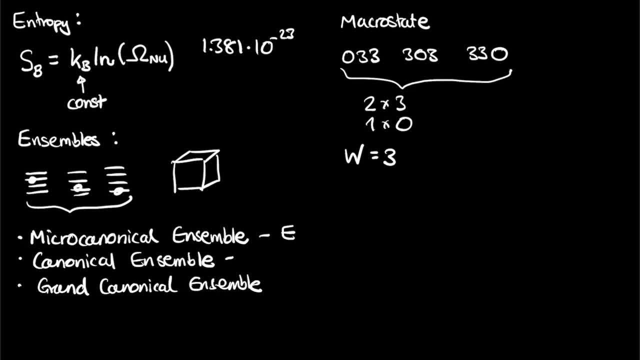 this is a macrostate, Simple as that. So it's kind of like a way of grouping together certain atoms, certain molecules, pretty much, And the probability of it being in a particular macrostate rather than a microstate is, rather than one, over omega. it's w. 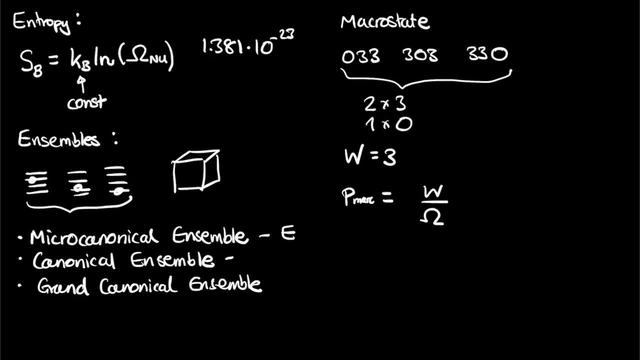 Over omega. So what's the probability of it being in this macrostate right here, this collective macrostate? Well, w is three and omega is 28.. So we can see that the probability of being in this macrostate is three divided by 28, in this case, right here. 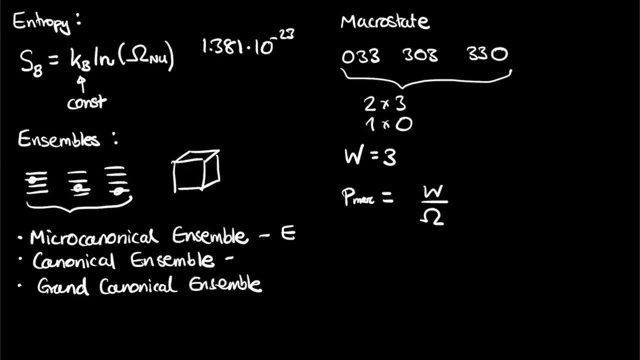 So that is what a macrostate is. It's basically a way of grouping together microstates. Now you can probably imagine that macrostates are pretty hard to kind of label and quantify. The way we do it is, we specify a macrostate by the occupation number. 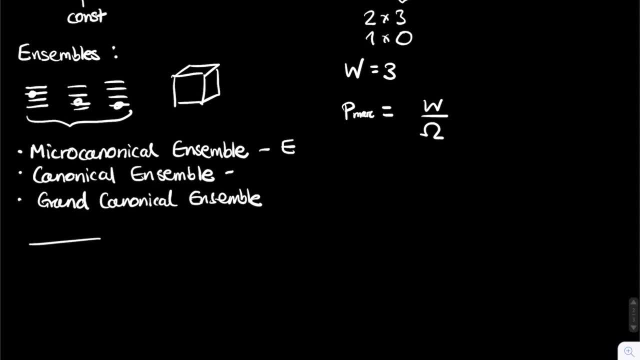 of each state. So let's just draw it out, just so we know what we're talking about. So here's our set of energy levels yet again, And let's carry on with this macrostate of two, threes and one zero. So we have one zero and two threes right here. So this is zero: one, two. 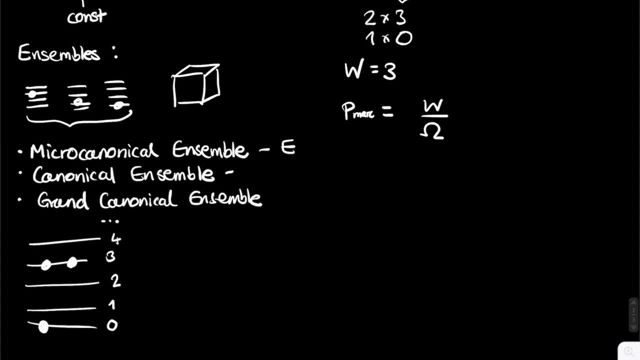 three, four and so on and so forth. So this is a macrostate right here, But of course we have three different microstates for this macrostate, And so the way we write this is that the number of particles in energy level zero, which we denote by the symbol n naught, is equal to one. 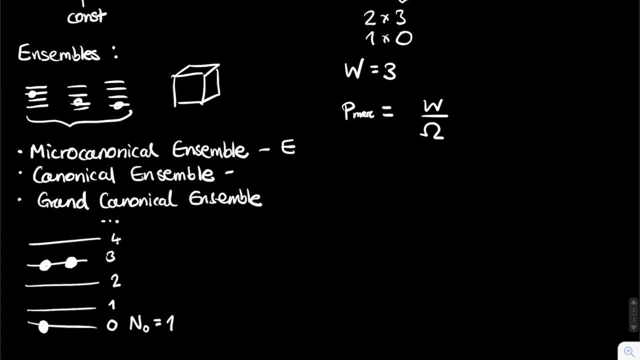 So this is the number of particles in the bottom energy level. So this little subscript here is the same as this energy level right here. But this number here is just the number of particles in that particular energy level, in this particular macrostate. So that is n naught. 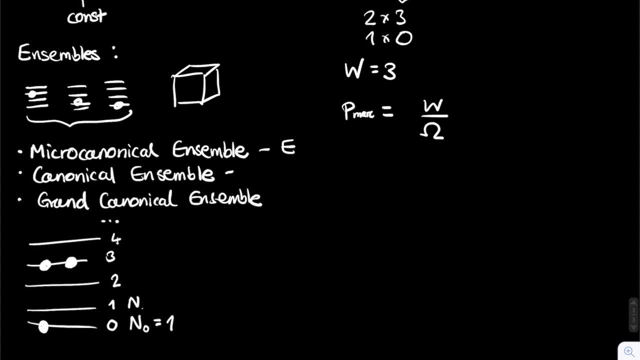 Let's just carry on and go through them, just so we're very clear about what we're doing. So how many particles are in energy level one? Well, zero. How many particles are in energy level two? Again, zero. But what about energy level three? 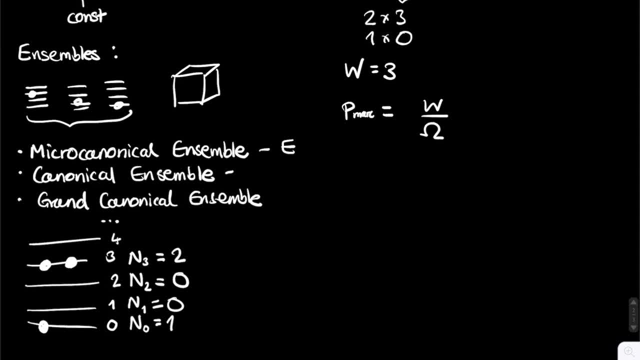 Energy level three. we can clearly see that there are two particles in this one, And so well, there we go, We've used up all three particles, And so with our n equals three system, then we have done them all, so we can. 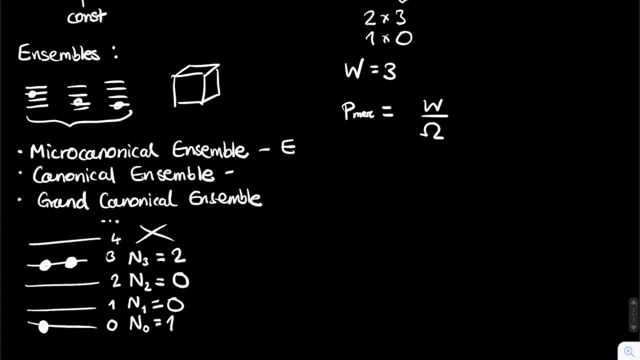 assume that there's nothing more in the rest of these energy levels. So that is how we denote a macrostate. We denote it by the occupation number. So we can simply write that n is simply the sum over j, where j is the energy levels right here from j equals zero to some point j you know. 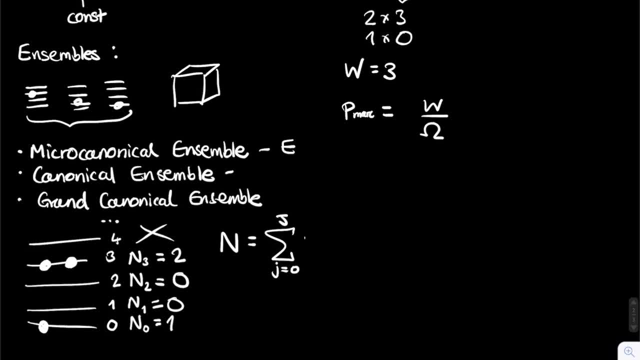 it could be infinity, it might not be infinity, you never know of nj right here. So in this case we've got it to write one plus zero plus zero plus two, So that again is equal to three, which is of course the number of particles that we have. So all is well so far. 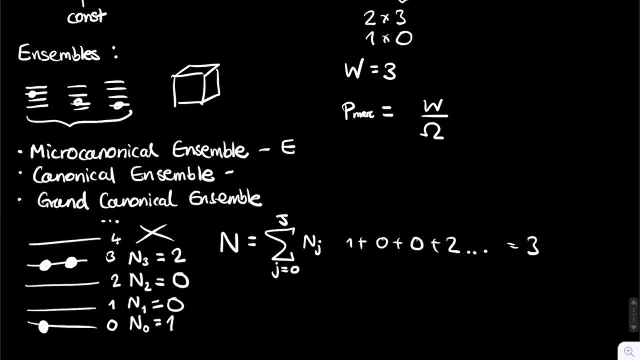 All is well. So that's n. What about the energy u? How can we work out what this is from in this simple example right here? Well, we said that the n is three and u is six before. So how do we show that it's six? Well, u we simply write as the sum. 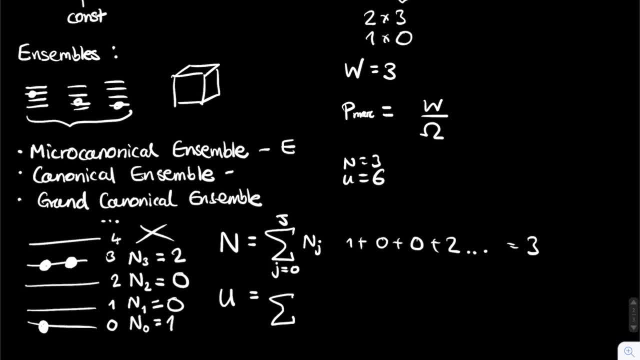 it's. the total energy in the system is the sum of the energy value multiplied by the number of particles that are in that particular energy value. So sum of ej multiplied by nj, It's simply the sum over all of the different energy states weighted by the number of particles that are in the energy states. It's a very common thing. 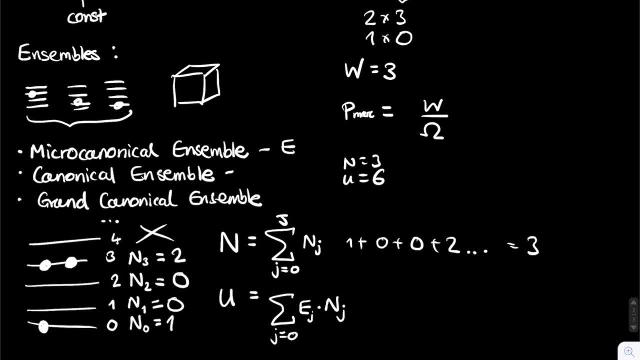 that you'll see quite a lot. So this is a sum from j equals zero to j. Again, we don't know what j is. it could potentially go on forever, but in this case we just got nothing after this point here, nothing higher than the three level. And so what would this be? What would we get? 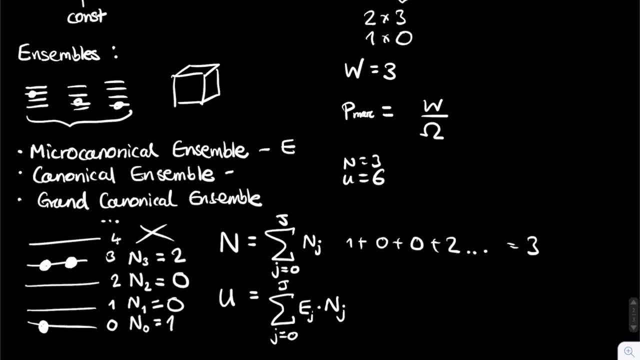 if we expand out this sum, Well, if we've got one particle on the zero energy level, that's not going to contribute anything. So we've got zero n equals one level, no particles, so that's just going to be another. zero n equals two level, no particles, so just another zero n equals three. 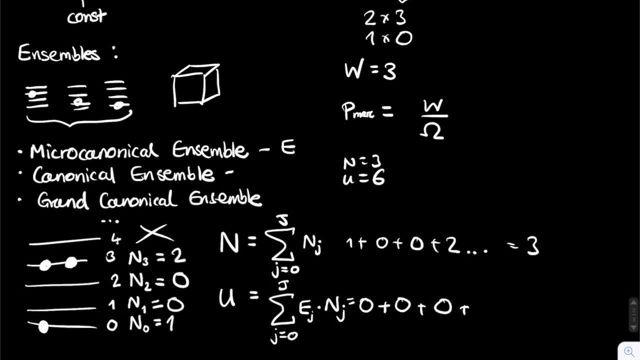 level. oh well, the energy of the n equals three level, is, well, three. this is the energy. three, the third, the three level, if you like. and how many particles have we got? we got two, and so that is just gonna equal six, which is the amount of energy that we had. so all is well, all is well. 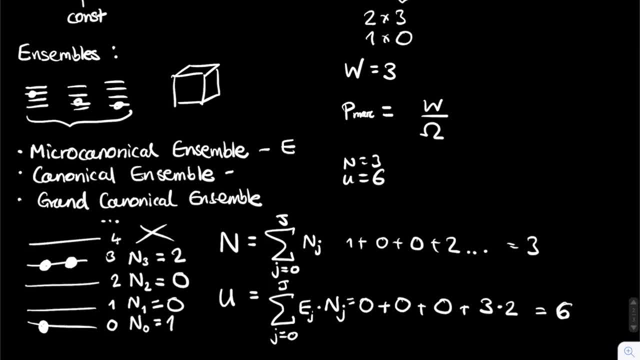 we can derive what n? u is if we know, if we have this sort of state here, we know what n and u is, and these formulas are quite important and i'll so. therefore, i will just put a little highlight around them. and there's just one thing that i missed out, and that is basically how did i work? 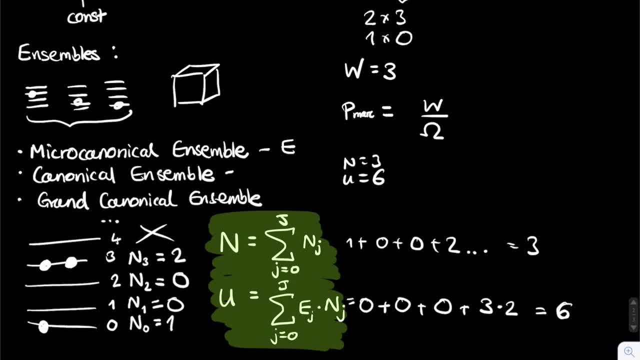 out that there were three microstates. for this particular macro state right here, well, um, w, right here is simply: n is simply equal to uh n, which is the total number of particles. in this case, it's three factorial divided by now. this is where it gets a little bit weird. uh, we're going to have a sort of 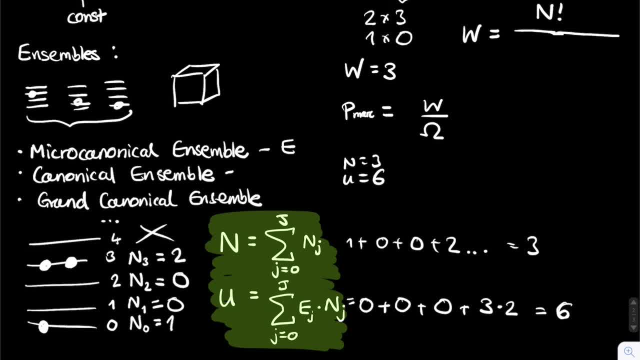 an infinite product, uh, basically, and we're going to write n naught factorial multiplied by n1 factorial, multiplied by n2 factorial, n3 factorial, and so on and so forth, right the way up to, uh, the infinite energy. but, as you're hopefully aware, zero factorial is equal to one, so don't. 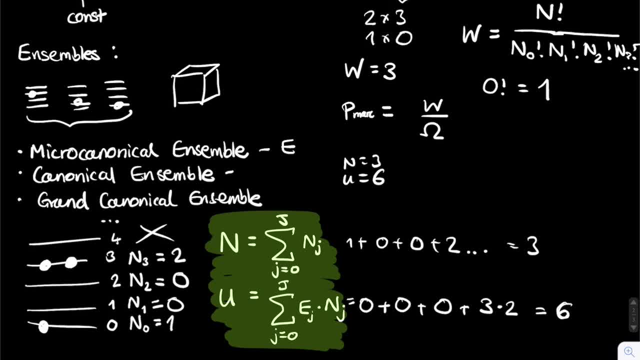 worry about this whole divide by zero problem. it's not a problem because we've- we've put a factorial in front of it and so therefore, um, any zero terms in the denominator right here will just go to one, and so, uh, how do we, well, how do we work this out? so we've got um. so in this case, 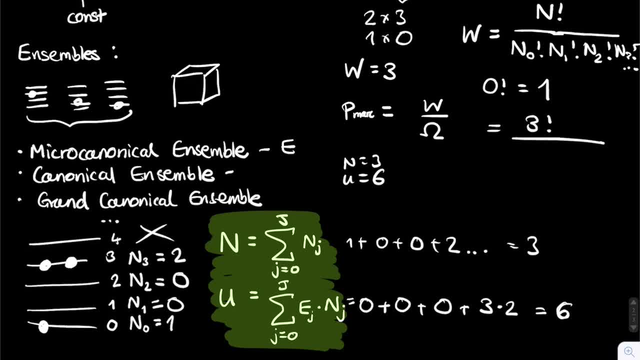 we've got zero factorial with zero factorial and we've got zero factorial here, so we're going to have three factorial on the top. there is one particle in the zero state, so we're going to have one factorial there. nothing in the end in the one state, nothing in the two state. 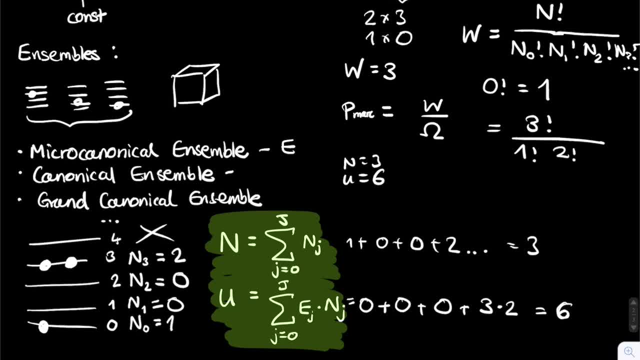 but we're going to have two particles in the three states, so therefore it's two factorial as well. so these are multiplied and we're just going to get one for the rest of these, and it's going to be an infinite number of zero factorials, and no matter how many times you multiply. 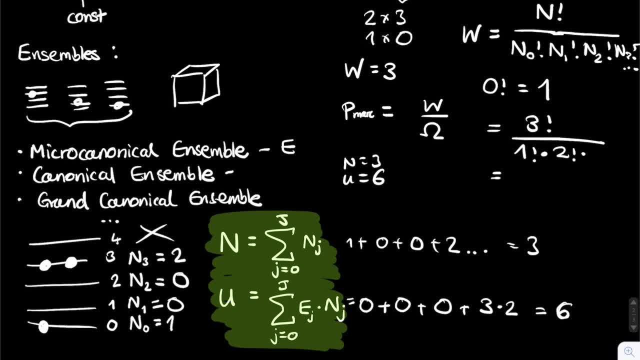 by one, you're just still going to get one. and so what's this? well, three factorial is six divided by two. factorial which is two, which equals three. so this is a handy way of calculating the number of microstates per macrostate. um, we often give this term w? uh the label, the macrostate multiplicity. 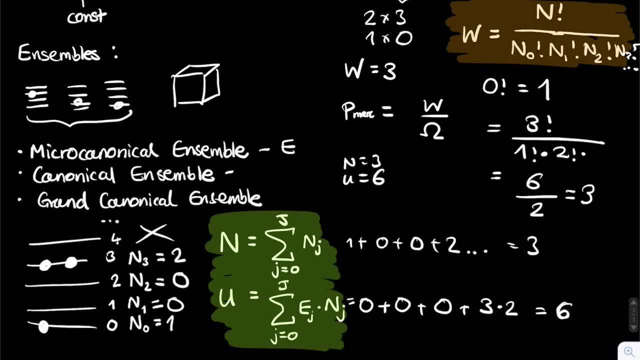 um, so it's the. it's the number of macrostates, the number of microstates for a given macrostate, and i hope that makes sense. so on to the next bit.